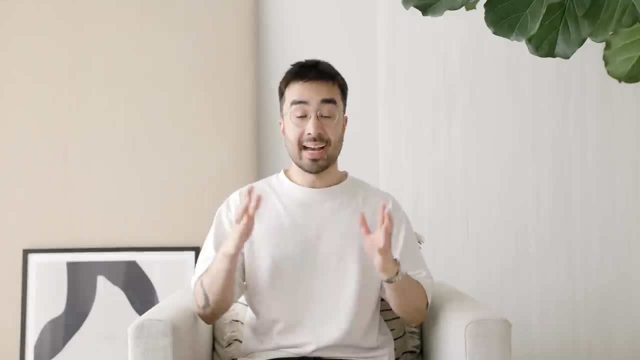 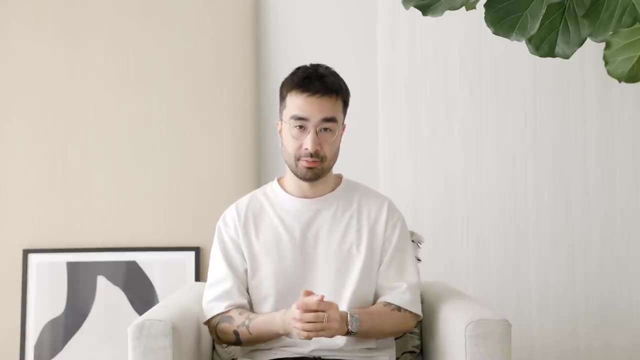 a red tie to evoke a feeling of authority. Also fun fact, it is actually the first color per seed by the human eye when you're still a newborn baby. It is a highly energetic color and is considered to be a physical stimulant. It stimulates our senses of smell. 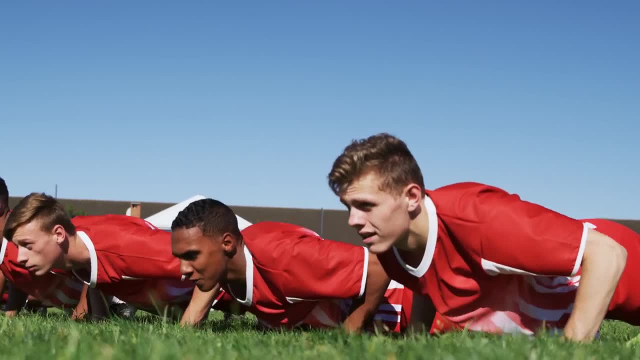 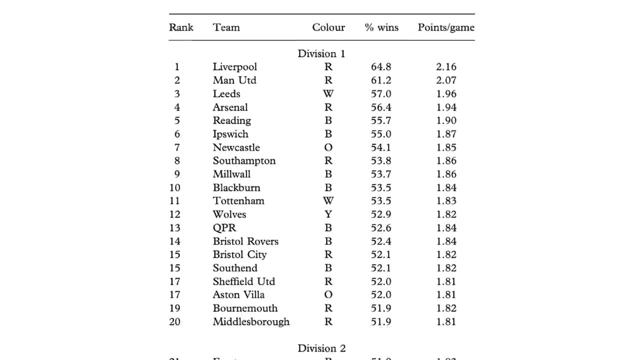 taste and our adrenal gland, which makes us more prone to take action and gives us more energy. In fact, scientists from Plymouth and Durham University analyzed the winning history of 68 top English teams from 1946 to 2013, and they found that, regardless of experience, the teams 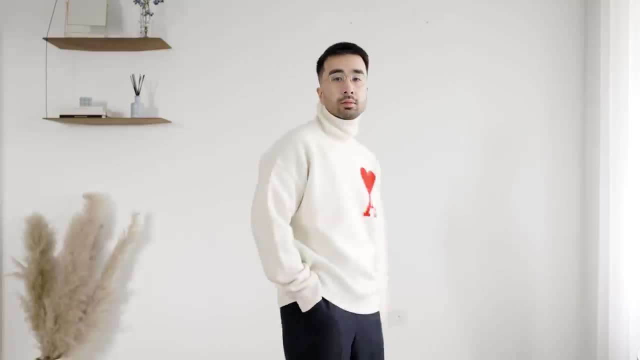 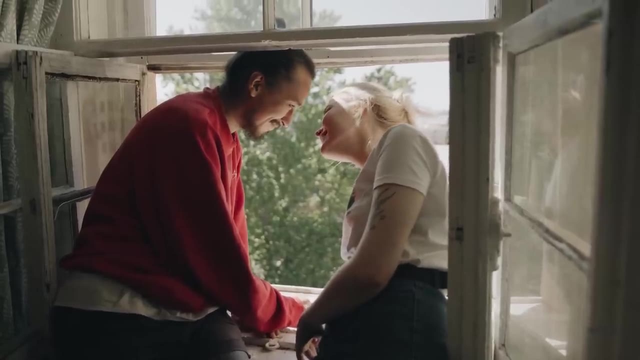 who wore red win more than they lose. It is definitely an attention-grabbing color. Wearing red shows that your bold, confident and are comfortable being the center of attention. It can be a powerful choice of color for a first date, but the downside is that it can be perceived as quite aggressive. 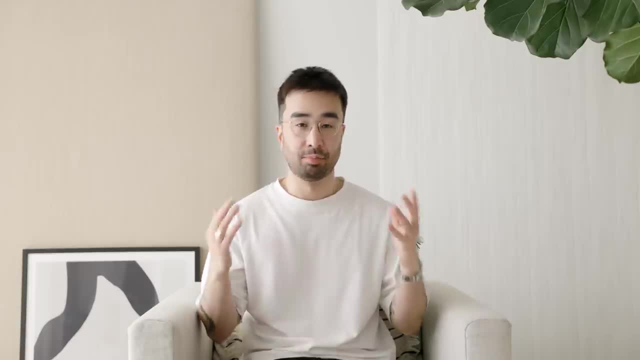 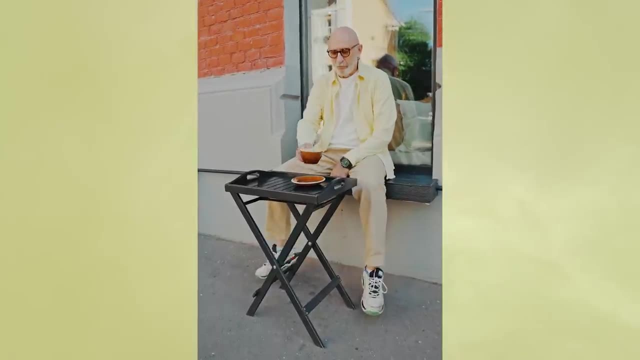 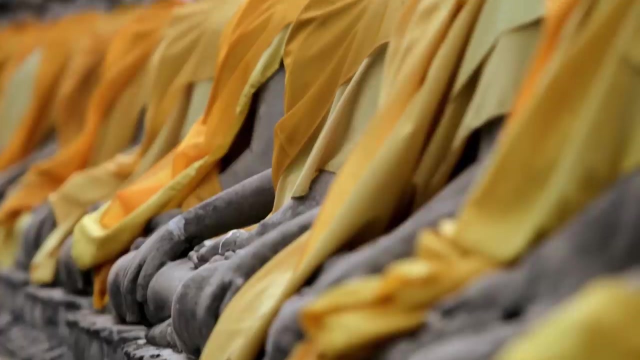 Ah, yellow, The happiest color of them all. Yellow is the bright, cheerful, younger sibling in the color spectrum. It represents happiness, creativity and positivity. It is a youthful color that is often associated with energy and curiosity. Interesting fact, it is often used in Buddhism, where it holds a different meaning. It is a symbol of humility and 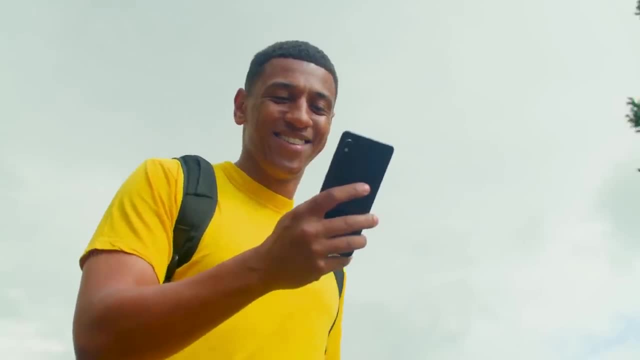 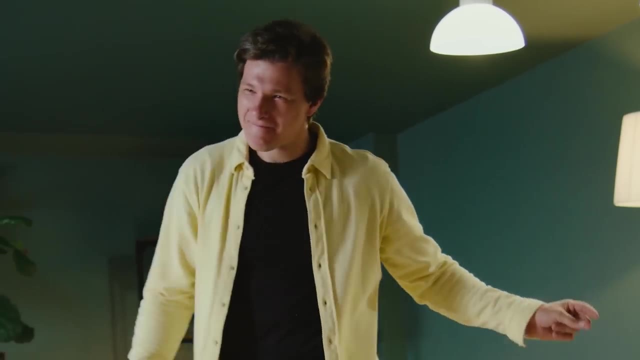 inspiration from a materialistic society. Wearing yellow can make others perceive you as energetic, creative and curious, and it can make you feel more joyful and optimistic. On the downside, though, you can also be seen as not so serious, so you want to be careful with where and when you wear yellow. 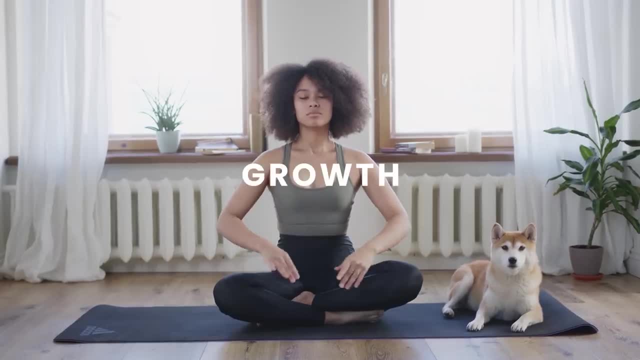 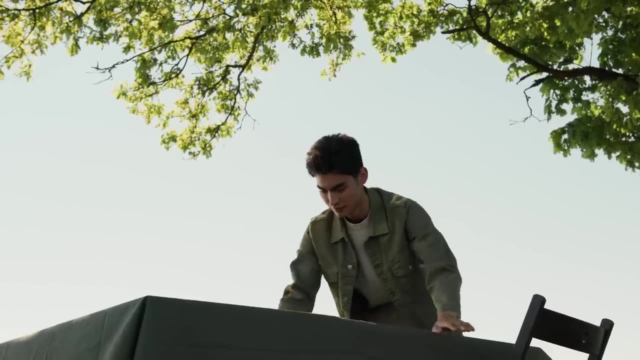 Green. Green is known to be the most calming color. It represents growth, balance and health. Whenever you see a lot of green in nature- trees, plants, greenery- it is a good sign of health and an abundance of resources, which is why we often associate it. 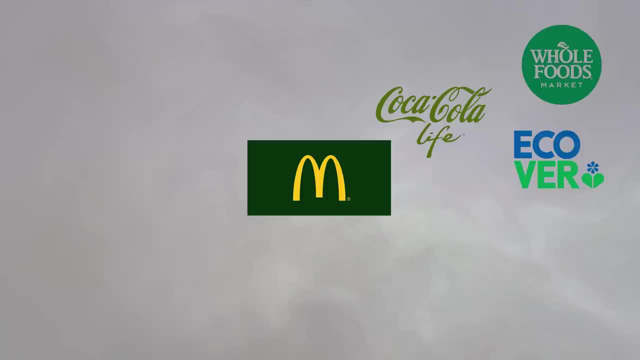 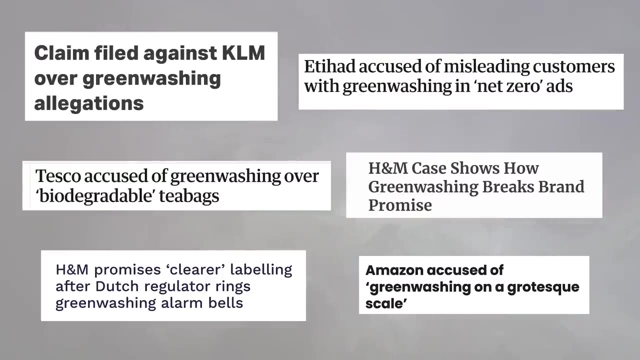 with prosperity. It also gives a feeling of eco-friendliness, which is why companies who want to communicate sustainability often use green in their branding. Unfortunately, that doesn't always mean that they actually are eco-friendly. Wearing green can make you feel more grounded. 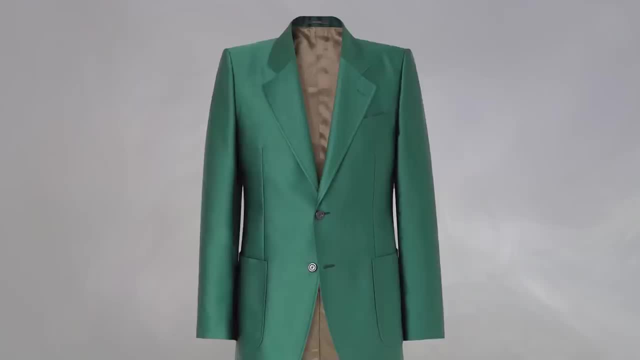 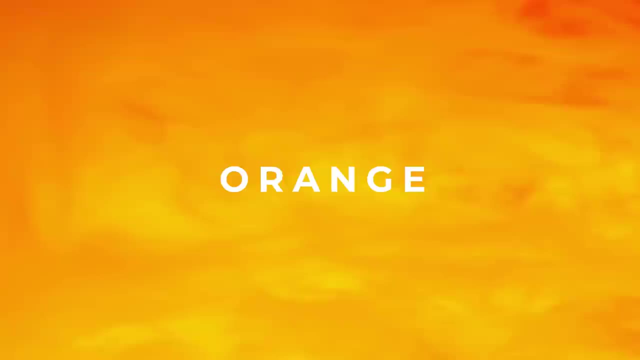 optimistic and less stressed. But the wrong shade of green for your skin tone can look unflattering, so you want to make sure that you pick a green that suits you. Let's get into some of the secondary colors now. Orange is the mix of red and yellow. It 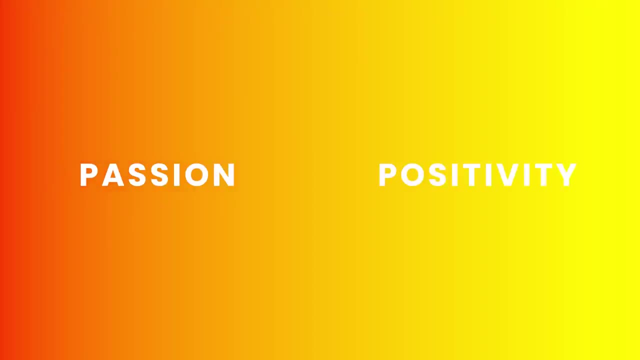 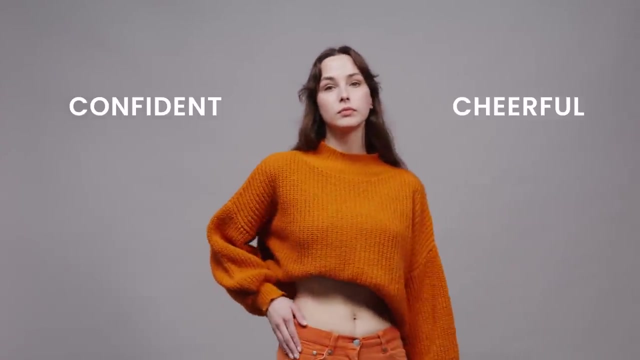 is an interesting color that holds the passion of red and the positivity of yellow. Orange represents enthusiasm, warmth and playfulness. Wearing orange can make you feel more cheerful and confident, But when it comes to fashion, it is also not the easiest color to pull off. 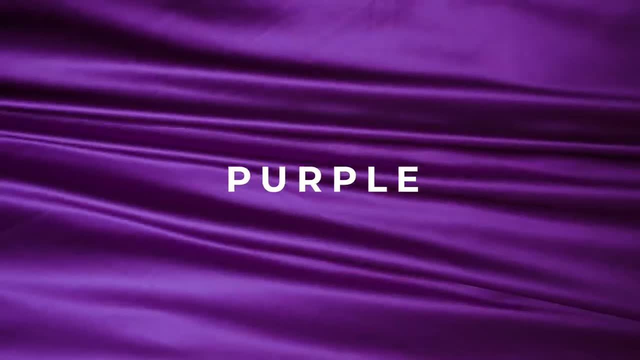 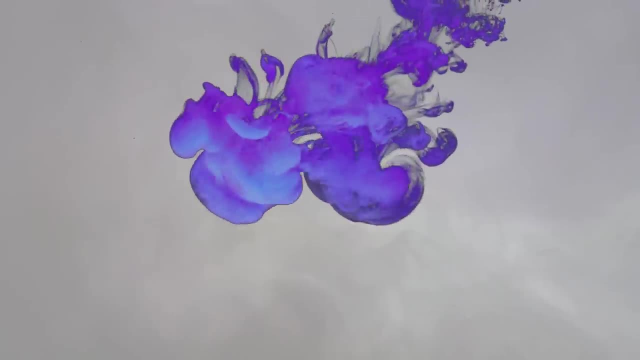 so wear it at your own risk. Purple Purple has many connotations and meanings. In the past it was associated with royalty and luxury, because the dye for the color purple was expensive and hard to come across, so only wealthy people could afford it. And to this day that connotation still. 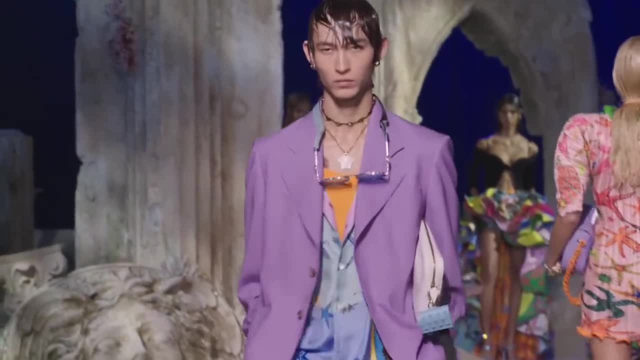 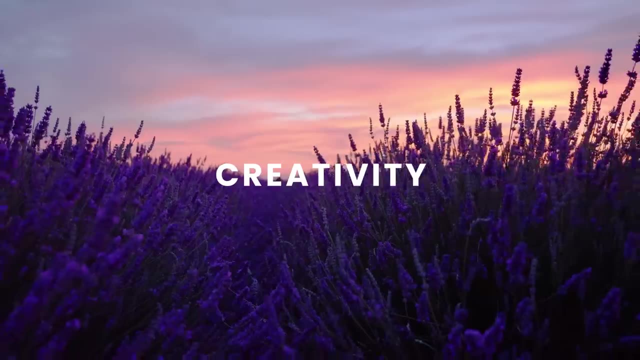 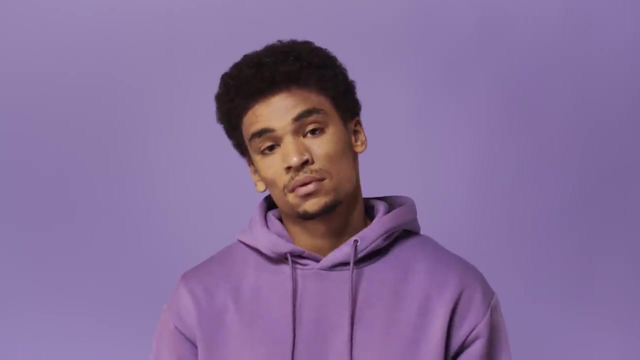 holds, as many luxury brands still use purple to evoke luxury. For example, Ralph Lauren named its most luxurious clothing range: Ralph Lauren Purple Label. Purple also represents mystery, creativity and spirituality. Wearing purple can make you feel more imaginative, help you think outside the box and you will be perceived as more intriguing. But 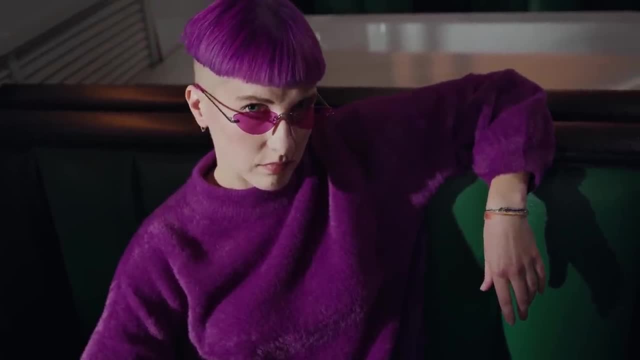 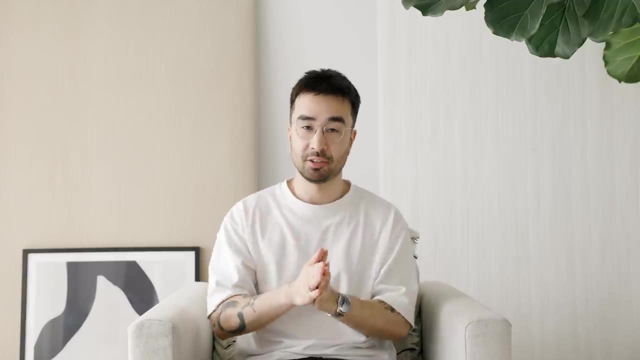 on the downside too much. purple can convey arrogance or quirkiness, sometimes not in a good way. But what about purple's younger sister, pink, Or shall I say brother? Today, pink is a color that represents compassion, love and femininity. However, in the early 20th century, 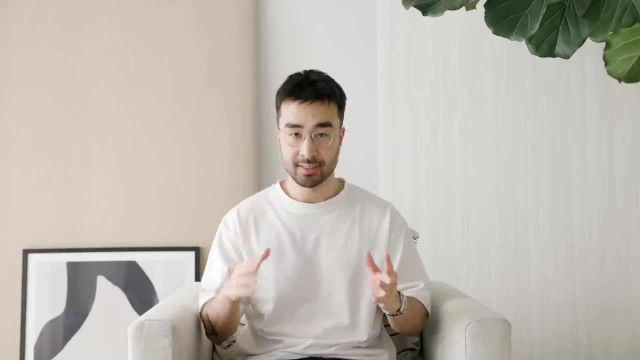 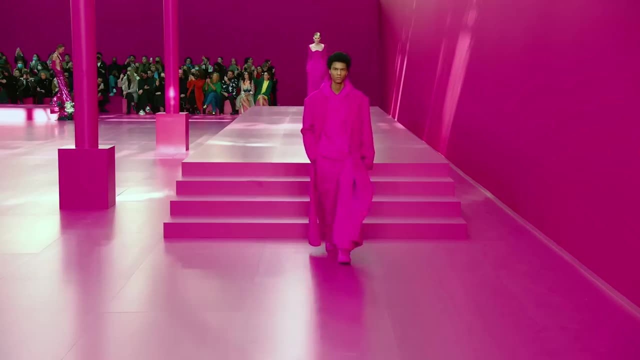 pink was considered to be a stronger color reserved for boys. Different shades of pink signify different things as well. The lighter, pale shades of pink are perceived as soft, tender and relaxing, while bolder, saturated shades of pink are perceived as energetic and 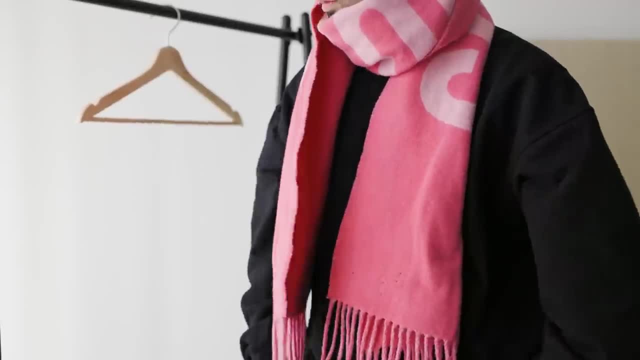 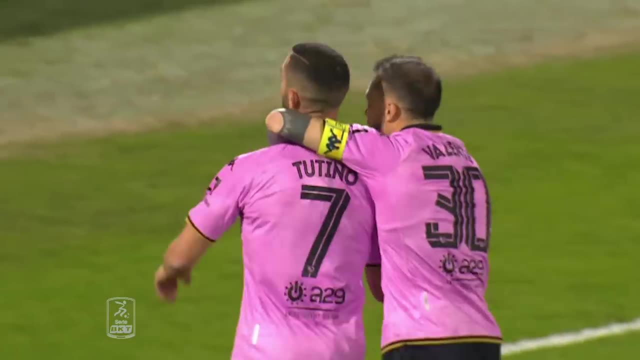 vibrant Wearing the color pink can make you feel more nurturing and empathetic, so if you're in a soft, tender mood, it can be a great color to wear. However, if you're about to do something highly competitive, like a sport, that requires 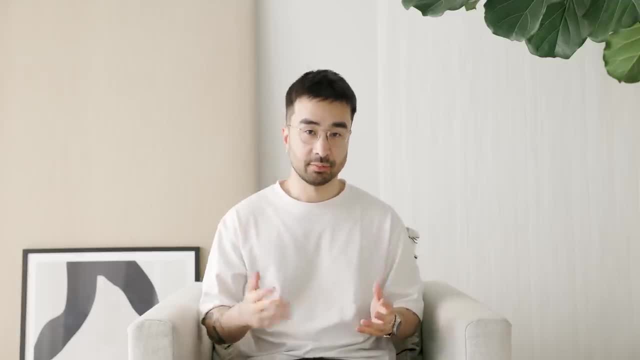 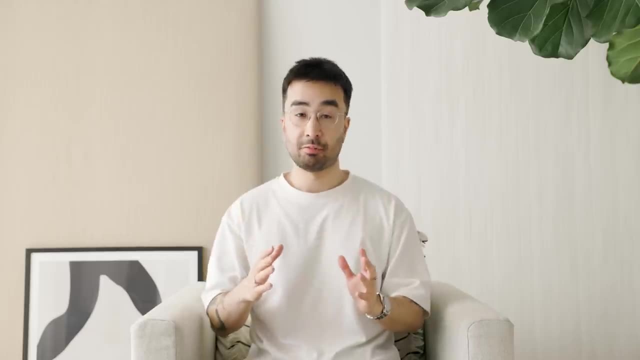 you to be at your peak physical performance. it might not be the best choice of color When it comes to fashion. many people love wearing black, myself included. It is a color that represents sophistication, elegance and power. Plus, it has the benefit of making you 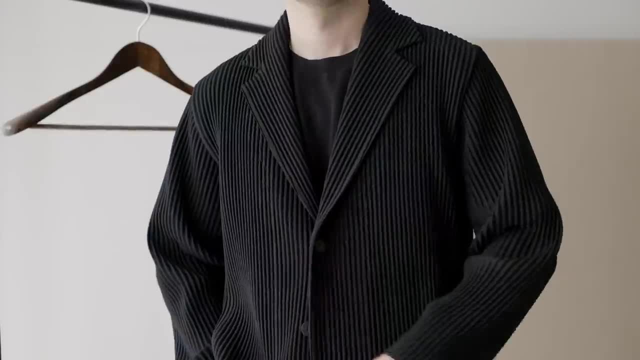 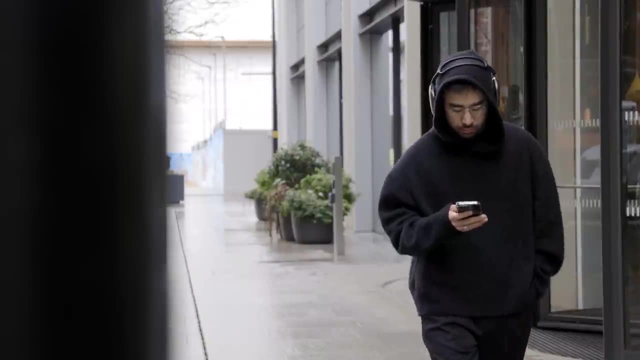 appear slimmer. It is a very classy, elegant color and also an emotionally safe color. You're not really putting out too much of yourself out there when wearing black, which is why many of us introverts feel good when wearing it, Also as universal of a color. 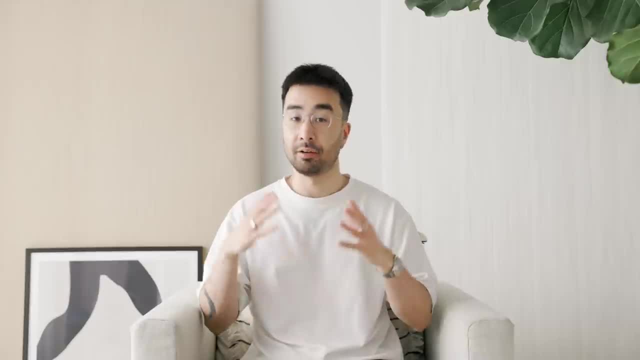 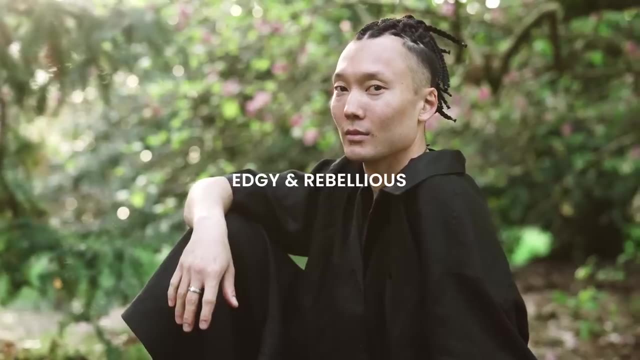 as black is, it can actually come across many different ways depending on how you style it. For example, you could be perceived as bold and authoritative, serious and strong, classic and practical, edgy and rebellious, or gothic and morose. 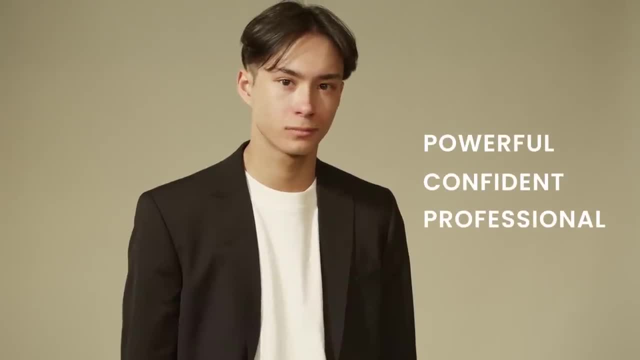 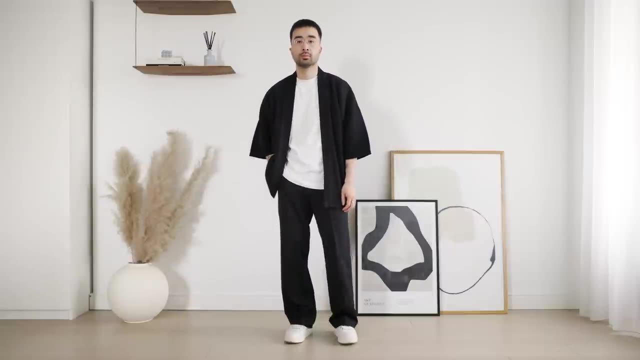 Wearing black can make you feel more powerful, confident and professional, But on the downside, constant exposure to the color black can negatively impact your mood. So maybe consider breaking up your black outfits with some lighter colors like white. See what I did there: Smooth. 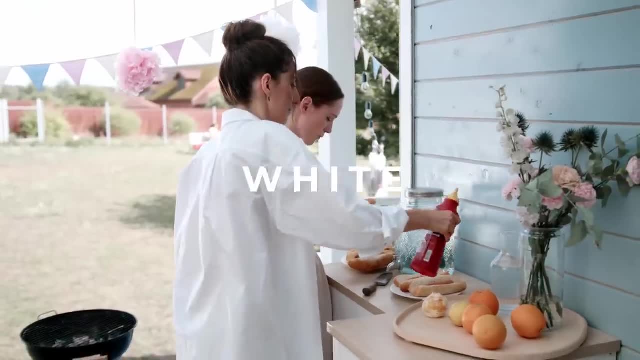 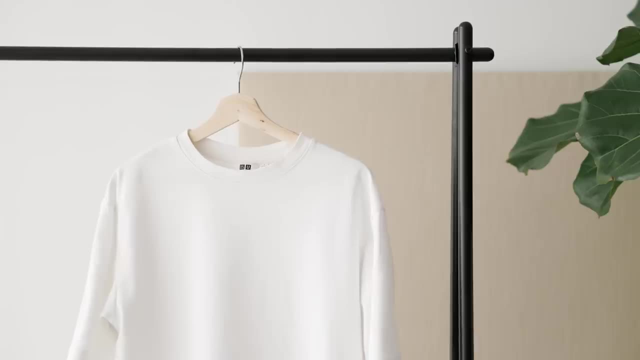 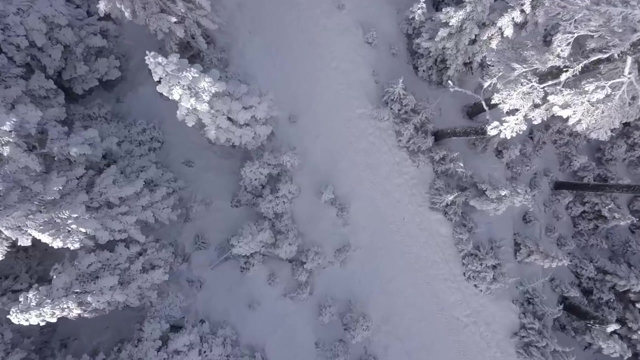 transition into white. Let's dive into it. White suggests that you're very careful with ketchup. Let's try that again. White represents purity, simplicity and cleanliness, which is why you can see white show up in clouds and the snow, both of which evoke a feeling of cleanliness and 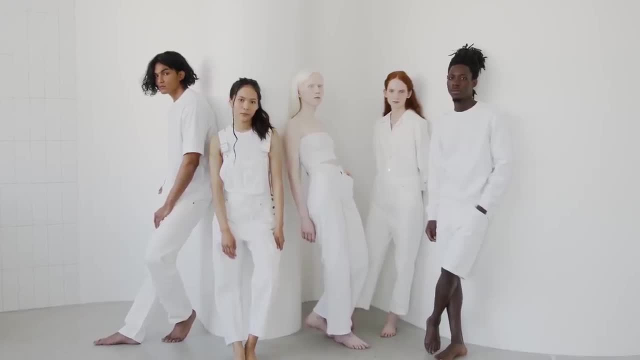 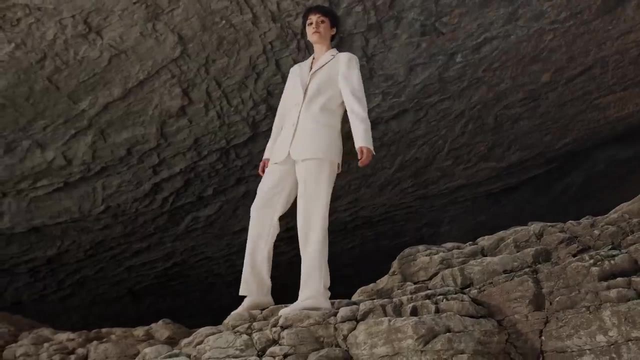 freshness. Wearing white will make you be seen as professional, elegant and clean, Like you've got your life together. It is often associated with new beginnings, so it is a good color to wear when you're starting something new and you just want a clean slate, a fresh start. 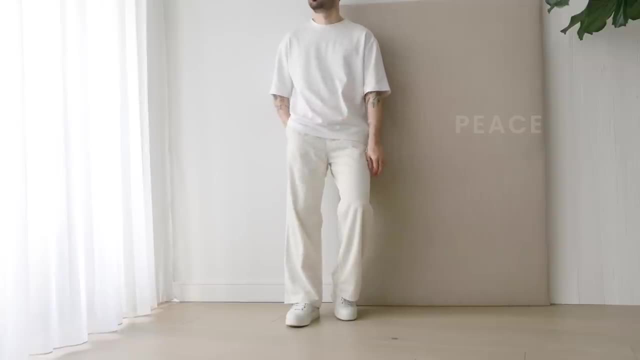 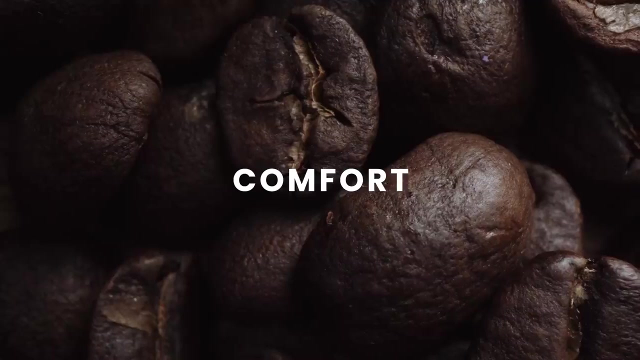 and you're ready to get your life in order. Wearing white will also give you a feeling of peace, calm and optimism. Brown Brown is linked to the earth. It represents stability, comfort and reliability. It's a very friendly, approachable color that will make people 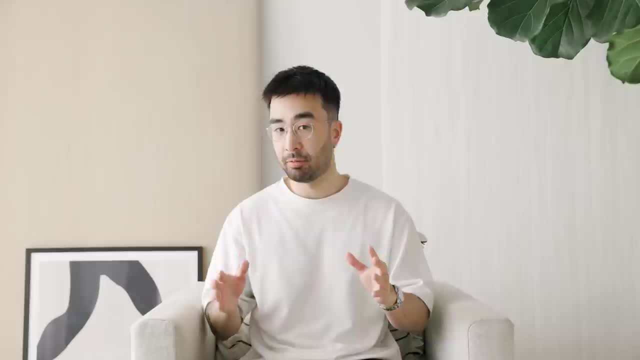 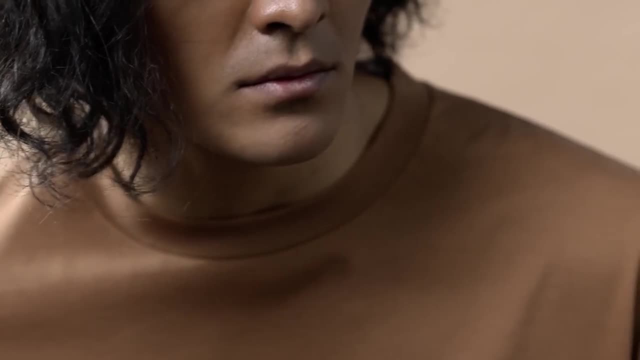 perceive you as warm, hardworking and dependable. It is a good color to wear when you're doing something that makes you feel slightly nervous, like an important work presentation. On the downside, though, it is a more mature color that can be seen as not very fun, or at worst. 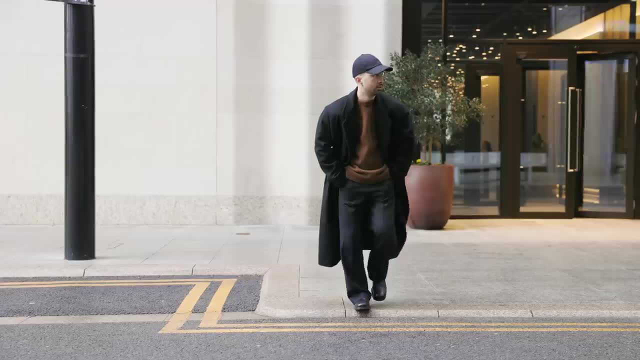 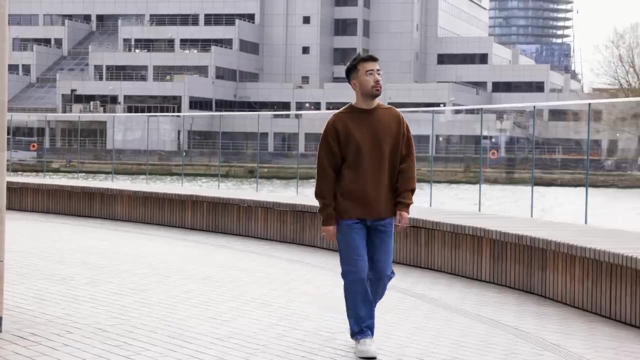 even boring. So it's good to pair with other colors to balance that effect. For example, a color combo with black can bring that sharp sophisticatedness to your look. Or blue naturally looks good with brown as it is a contrasting color on the color wheel and opposites attract. 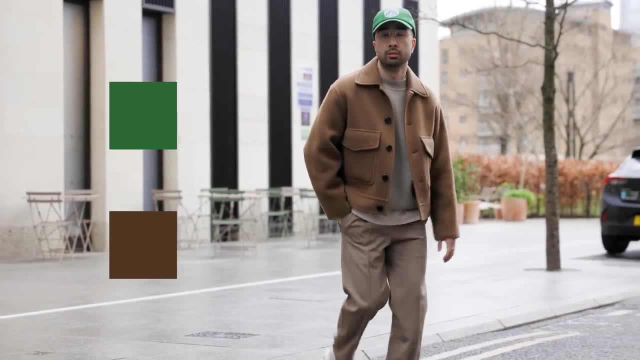 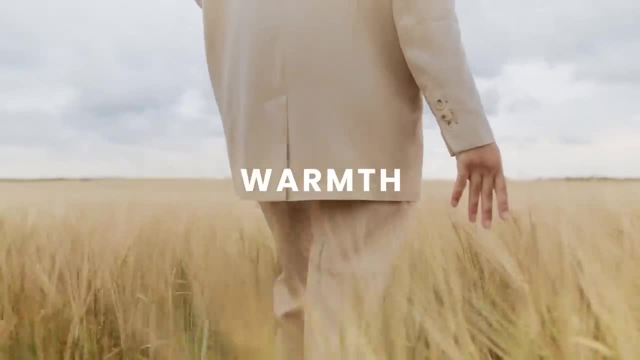 A natural fit with brown, leaning more towards that earthy color palette for a cohesive look. But let's talk about the softer version of brown, its wiser, younger brother, beige Beige, represents warmth, neutrality and calmness. It can be a very elegant, classy color when styled properly. 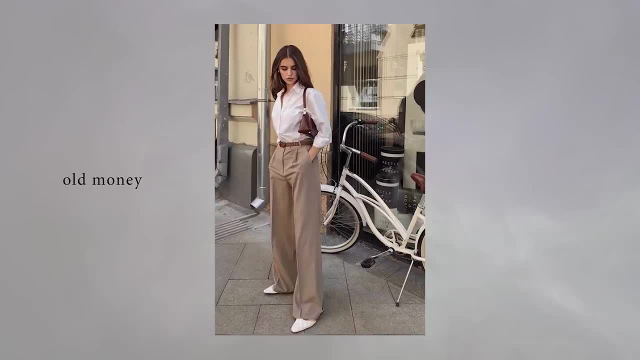 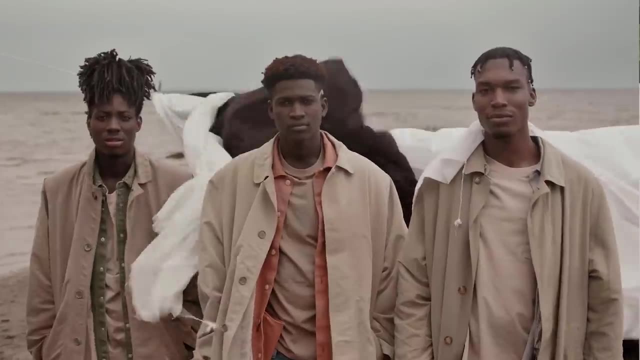 and it can give off that old money vibe that is so popular in culture nowadays. Wearing beige can also make you feel more relaxed and grounded. It is a very non-threatening, neutral color, so it's a great anchor to an outfit comprised of multiple colors, and it works especially well on. 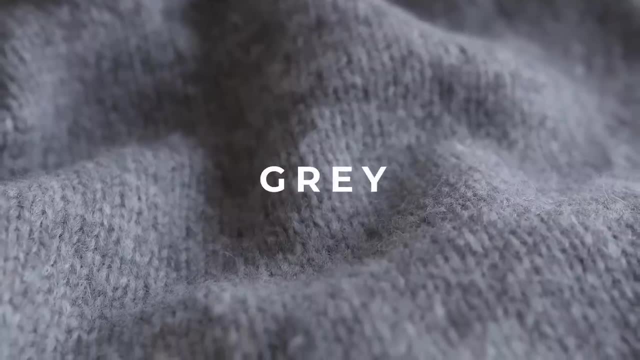 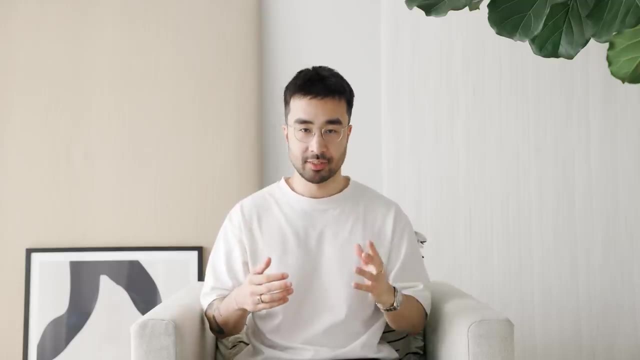 trousers and on coats. Lastly, we have gray. Much like beige, gray represents neutrality, but it also represents balance and sophistication. It's a very practical, non-aggressive color that is often associated with professionalism, formality and maturity. As such, it is often 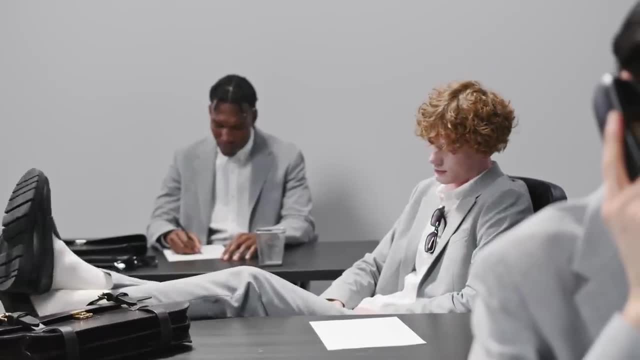 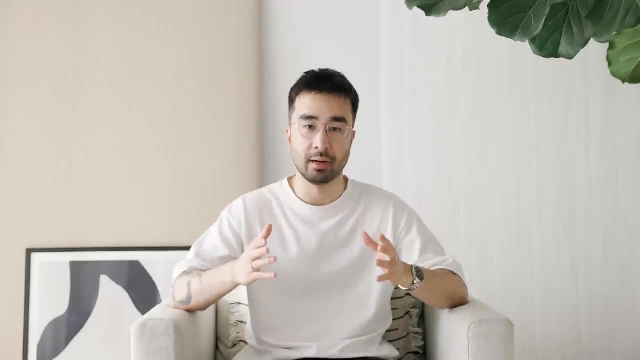 a favorite amongst business people for their suits. Wearing gray can make you feel more composed and professional and it can help you come across as an authority figure, like you've been in business for a while and you know what you're talking about. But on the downside, it can